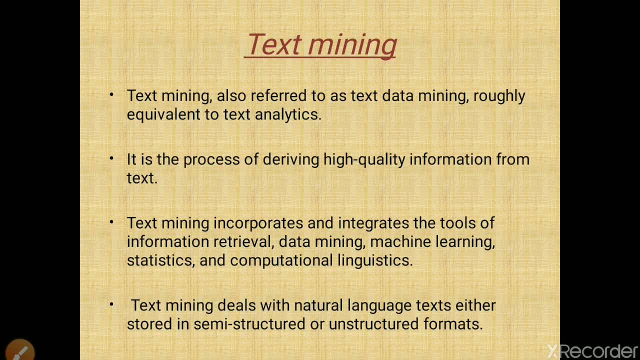 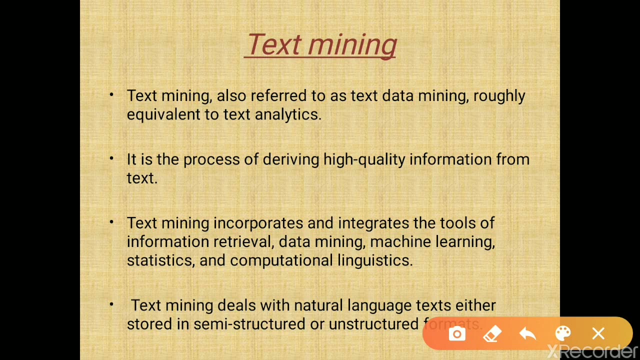 Text mining is. we will also call it as a text data mining. Text mining is actually the process of deriving high quality information from a text. So we are deriving a high quality information from the normal text, So we will call it as a text analytics also. One example, I will tell you: in call center transcripts, or in online reviews, customer surveys, and all from all this, we will mine the text that is present in that web page or any other text. 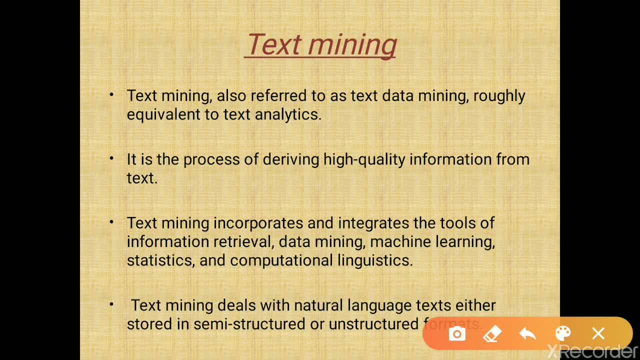 Any source and from all those we will get will get an idea. what about? what is about that particular document? Sentimental analysis for text and all is an example. So text mining normally incorporates and integrates the tool of information retrieval, data mining, machine learning, statistics and all, And data analytics normally use more tools included in statistics and text. data mining uses more tools. 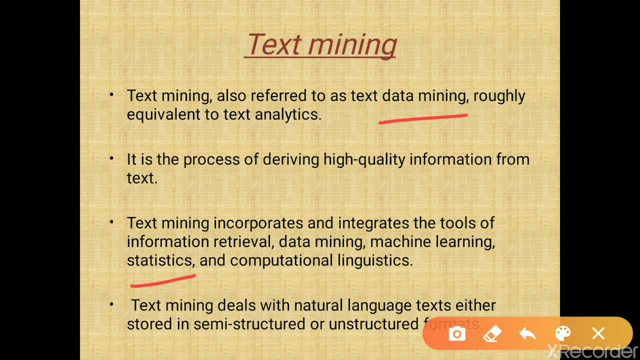 Concepts more related to data mining and text mining deals with natural language text either stored in a semi structure or an unstructured format. So once again I'll tell: text data mining is a process of deriving high quality information from a text which is similar to text data analytics, But in analytics we are using more statistical tools. So here we are incorporating and integrating tools of information retrieval, data mining and all in case of text mining. 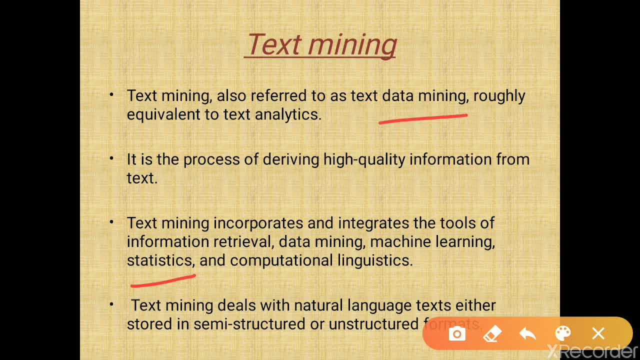 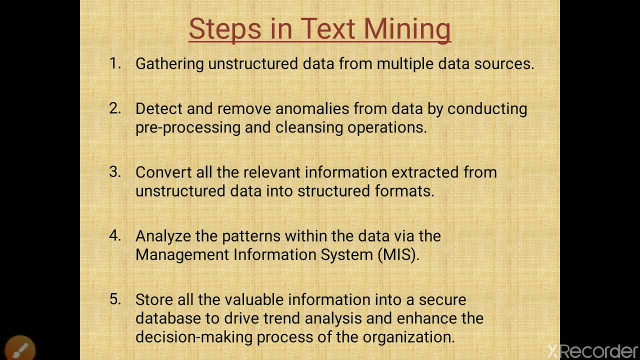 So if we are given with a text, we will mine the particular in particular text, what that text is giving, what information that text is given, that we will mine from that. Okay, so in text mining, the main steps in text mining are: gather, gather unstructured data from a multiple sources and detect anomalies. First, multiple sources are there. we have to gather the unstructured data. So the important thing is to gather unstructured data. 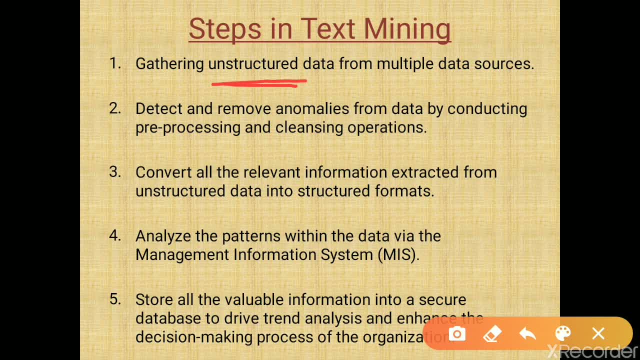 The second thing is we are gathering unstructured data from multiple data sources. What is the next step? Next step: we have to detect the anomalies and we have to remove it by pre processing in data cleansing techniques that we already discussed in our module one. So we are getting unstructured and impure data, We have to gather it and we have to pre process the data. So that's about the second step. Now what is the third step? Convert the relevant information extracted from this data. So the 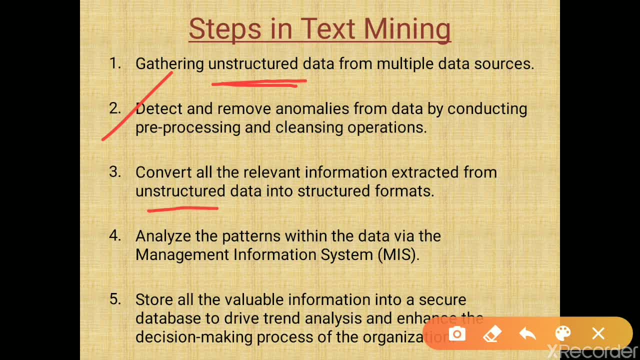 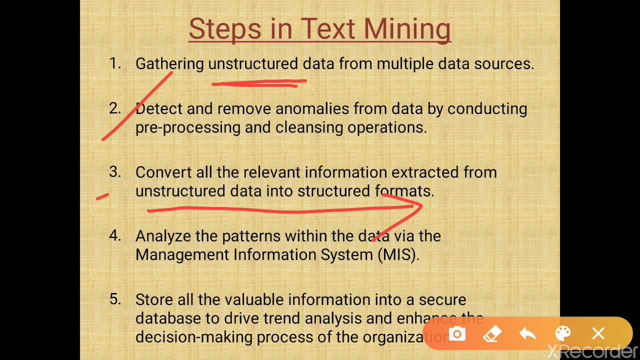 unstructured data into structured format. so third step is converting an unstructured data into a structured format. then next step is analyze the pattern within the data via management information system. so if we are given with a structured format data after the third step and this is given as the 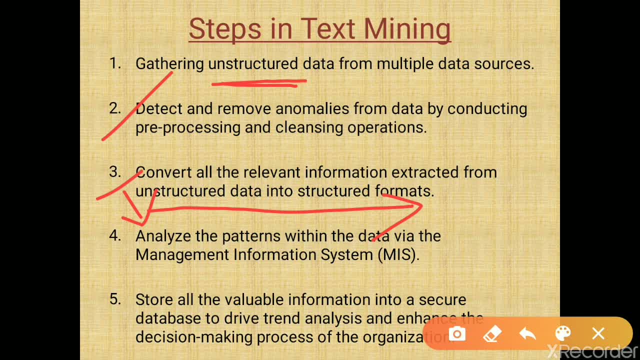 input for the next step from the structured data. we will analyze the data to find a particular usage pattern via using any of the techniques like management information system and all. next step is store all valuable information in the secure database to find the trend, to find the trend analysis and to enhance the decision making process of the organization. so these are: 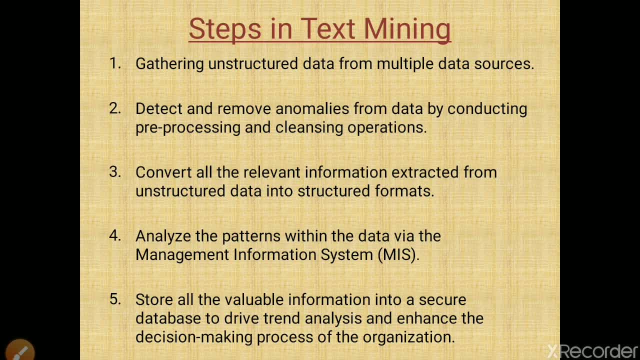 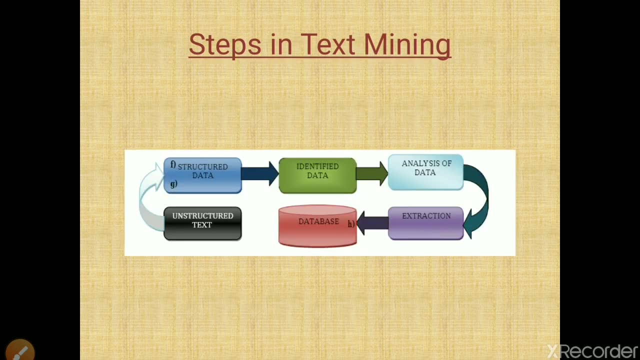 the main steps in the text mining. so we have to gather the data and we have to remove the anomalies. we have to structure the data, then analyze the data and store to find the pattern. so these are the main steps in that data mining. this is a schematic representation of steps in data mining. so first, 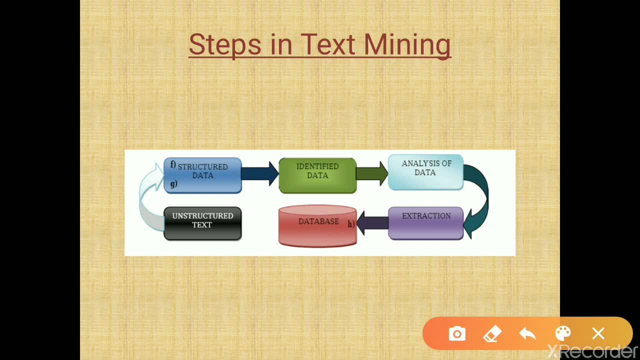 we are given with an unstructured data and this unstructured data. unstructured data is given, we have to pre-process and we have to convert in a structured format and we, after the structured format, we have to find the usage pattern right for identify the data, where we have to analyze the data and will extract something useful. 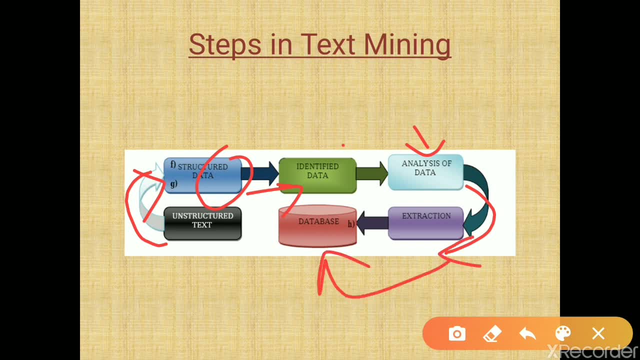 information from the data and it will be stored in the databases permanently. store the structured data to mine and to find the usage pattern or any interesting pattern for decision making process. so these are the main steps in text mining. next thing is the main text mining process, the process. 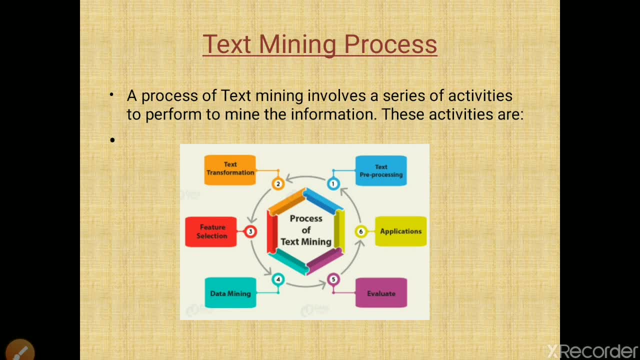 of text mining involves a series of activities to perform and to mine the information. these activities are text pre-processing, text transformation, feature selection, data mining, evaluation and application level. so these are the main steps in the text mining process. so we are familiar with all this process and all like text pre-processing and all we are very much familiar. 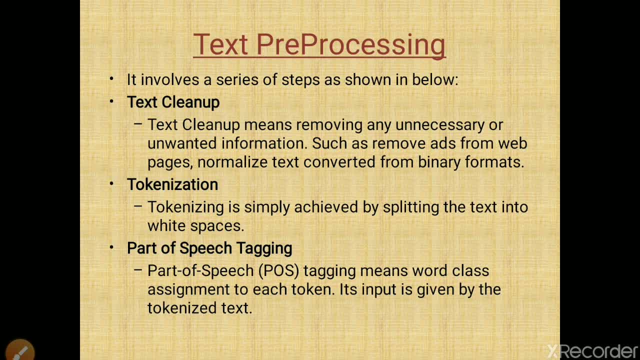 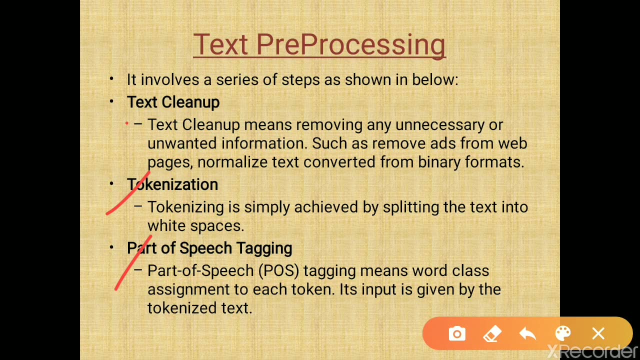 so what the text pre-processing will do. text pre-processing steps involves a series of steps like text cleanup, top text cleanup, tokenization, part of speech, tagging. so these are the main activities in the case of text pre-processing. so pre-processing your data means we will remove the anomalies and we will remove the errors and all. 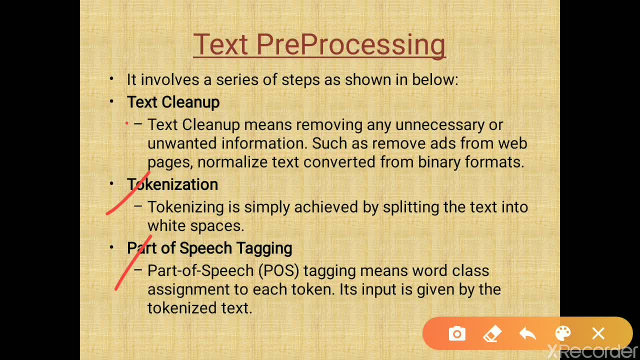 to get a pure form of the data. in order to get the purest form of data, we are removing the impurities in the data. that is known as text pre-processing. so here, text cleanup means removing any unnecessary or unwanted information, like an example is like removing add. 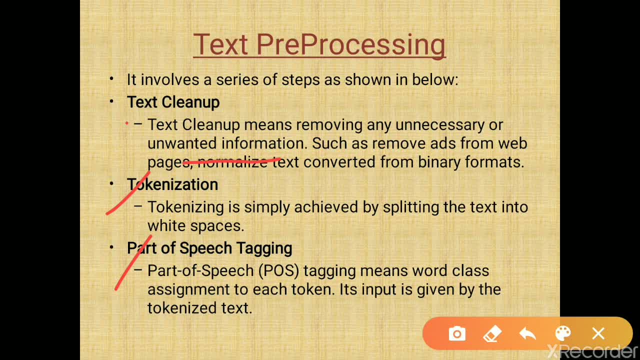 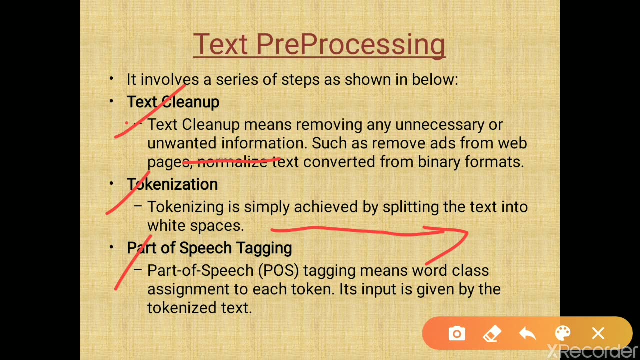 from the web pages or text is converted, normalize the text converted from binary format, or some examples for text cleanup. now what does mean by tokenization? we are given with a sentence. we have to split the text into tokens. tokenizing is simply achieved by splitting the text into white spaces. 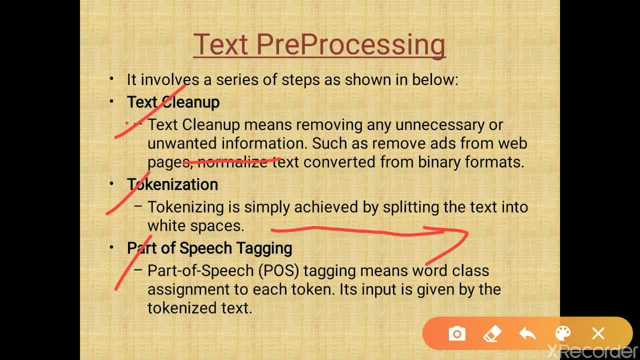 and all. so we will mesa, stop, stop, stop, do cap, make it into tokens. So after getting the tokens we have to tag it with the part of speech tag right. POS tagging we have to do, and this is actually the world class assignment. 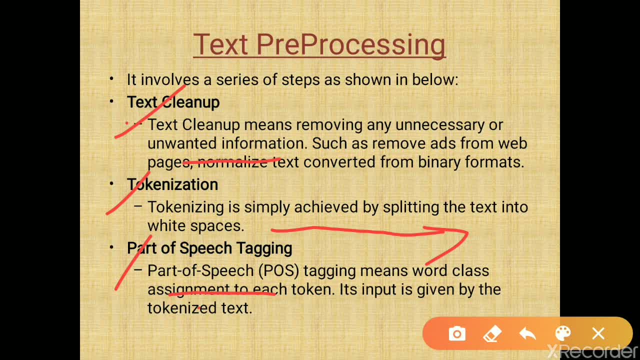 given, like if we are given with the sentence, we are divided into small, small token and each token represent what it is: it is a verb or an action or adjective. that part of speech tag will be added along with that for the tokenized text. that is the part of speech. 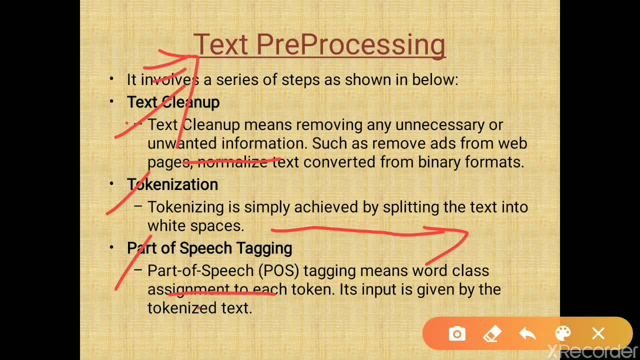 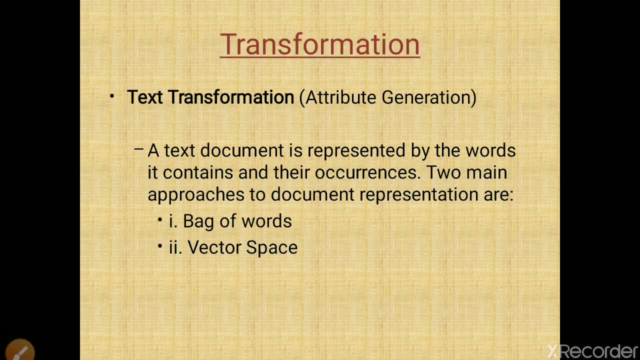 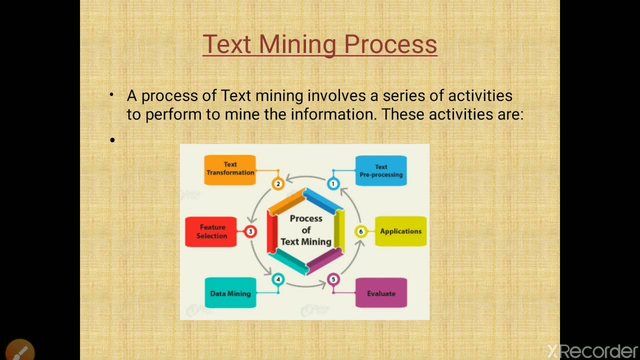 tagging- These are the main process- comes under text pre-processing. So in text pre-processing we will do the text cleanup, tokenization and part of speech tagging. Then after that, what is the next step in the text pre-processing? Next, after pre-process the text you have? 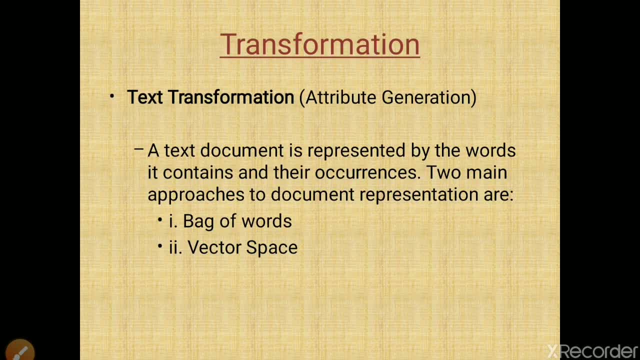 to do the text transformation. So what the text transformation will do, It is like we are given with unstructured. we have to convert into structured format, right? So this is the text. Just like an attribute generation, the text document is represented by the word it contains. 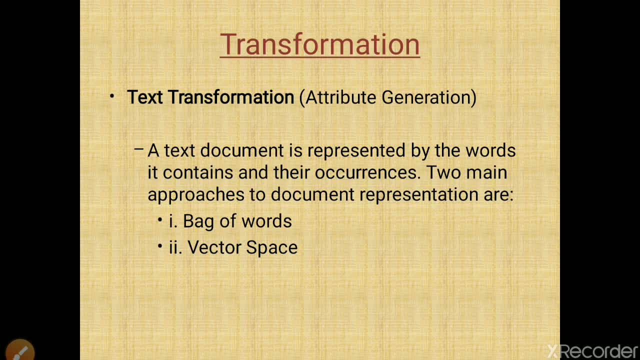 and the occurrence. Two main approaches in the document representation are bag of words and vector space. So these two, bag of words and vector space, is used for the text. document representation, document representation: What is mean by this bag of word, This bag? 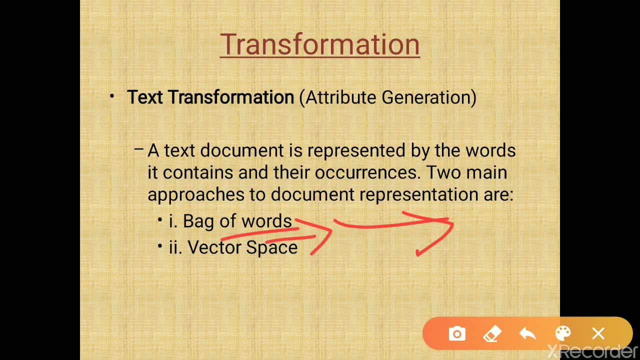 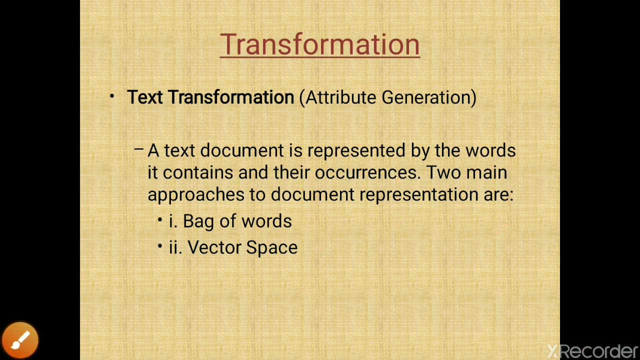 of word means. if you are given with some set of sentence, for example, hello welcome to. hello welcome to data mining- You will use those weapons in the text document that are mining studies. If this is the sentence, what ever it is like, we will divid it into tokens, right? Hello welcome. this is the sentence. 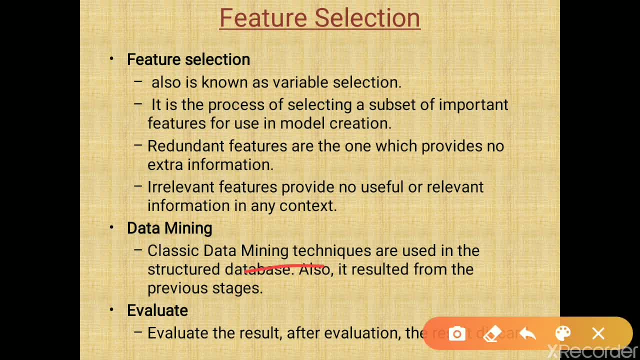 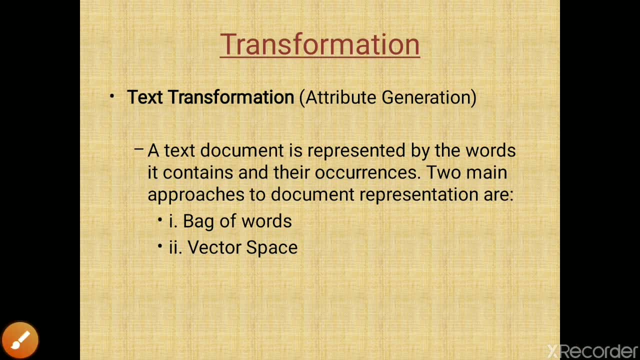 hello welcome is my particular sentence Or any other sentence. like a text document, is represented by the word it is. This is the sentence that I am constituting. What I will do is, it is like I will divide it to small tokens. 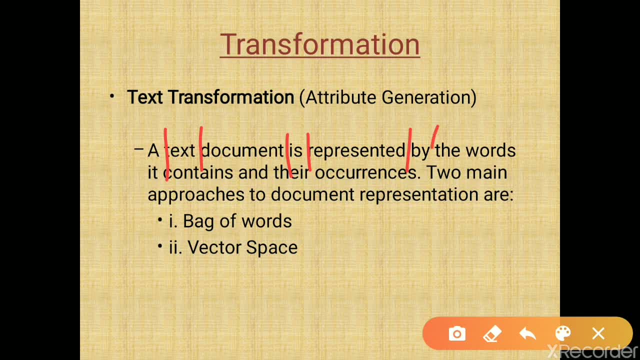 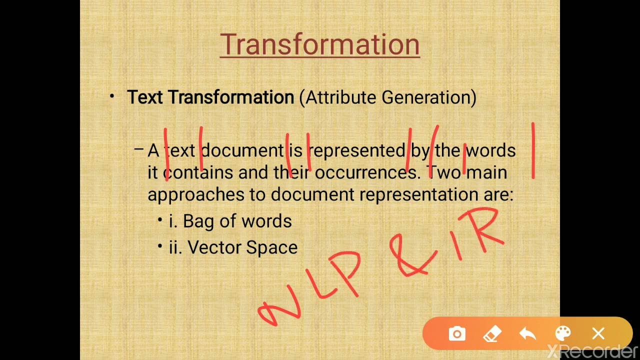 Say, cioè text document is represented by the words. So I'm dividing it into small, small sections and simplifying its representation by using NLP natural language processing and information retrieval process. Here the text is represented as a bag of its 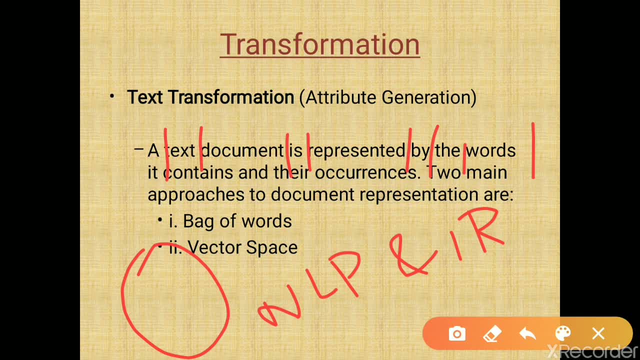 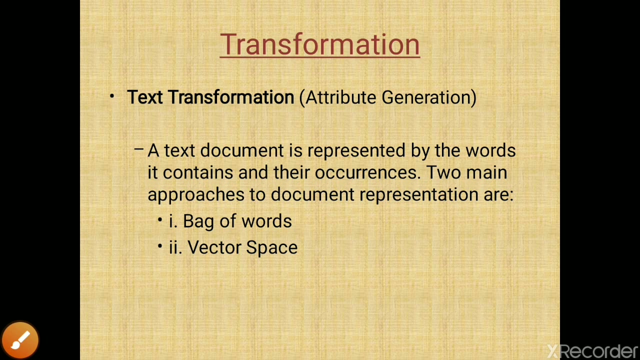 words, not considering anything regarding the grammar. So here I'll represent a text document is represented by the words. So each word, each document, each token is represented as a bag of words, not considering anything regarding the grammar. that is known as bag of words And in case of vector, 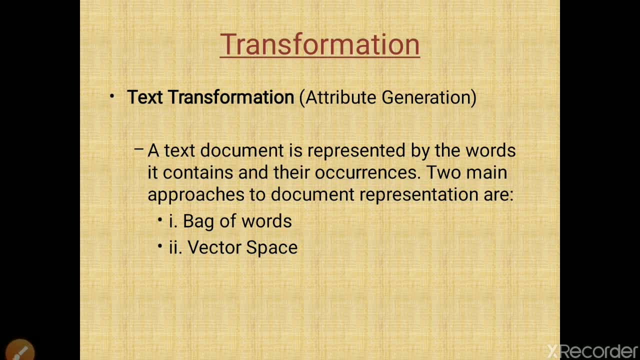 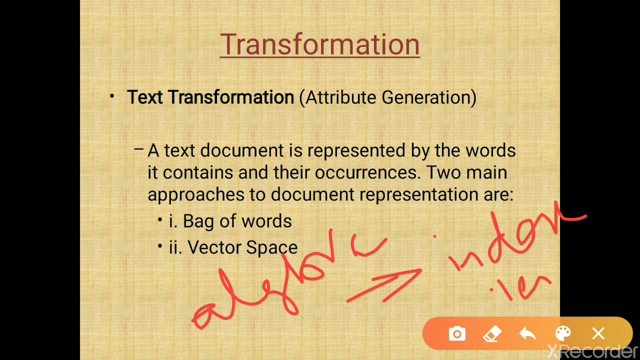 space. it is a document representation format. Here we are using an algebraic model. An algebraic model is used for representing a text document as a vectors of identifiers, such as index term that we are using in our system, and all is an example of vector space. So algebraic model of 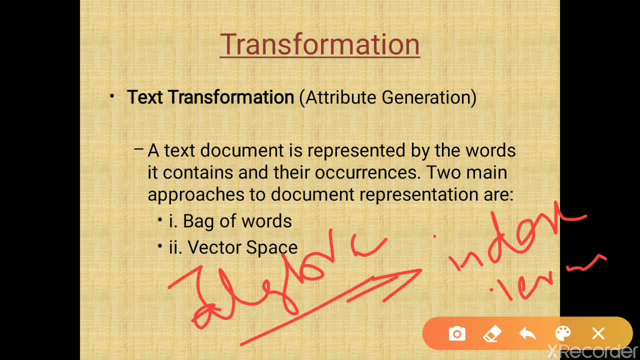 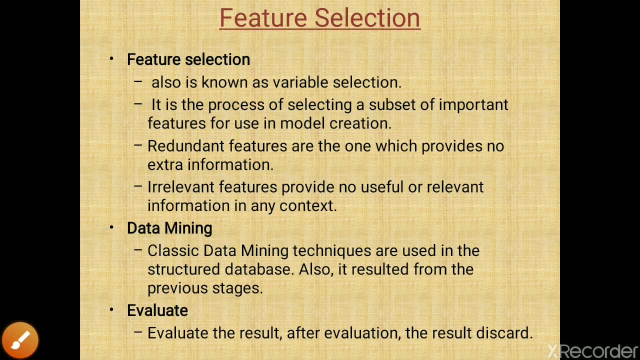 representation is a model representation of vector space is used in the case of vector space data representation. Here an example is index term. After the transformation the next step is feature selection. So feature selection is also known as variable selection. So index term is a variable selection process. It. 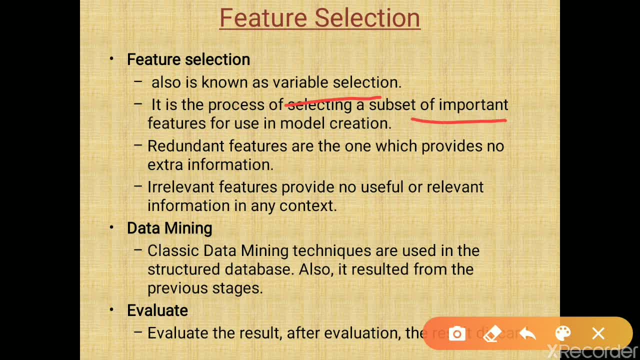 is the process of selecting a subset of important features from the model creation. So we are extracting the important feature. So what we have to do, while extracting the important features, we have to remove the redundant features as well as the irrelevant features. So these redundant and irrelevant features, 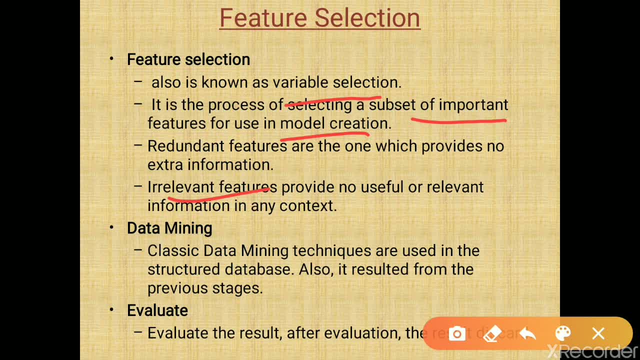 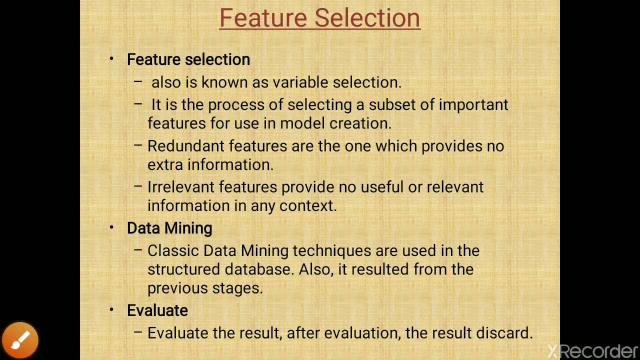 are not useful while doing the text mining process, So we have to remove it. Next is data mining. The classic data mining techniques are used in the structure data base also. it is result from the previous stage. Next, the next step is evaluation. the process Evaluate. 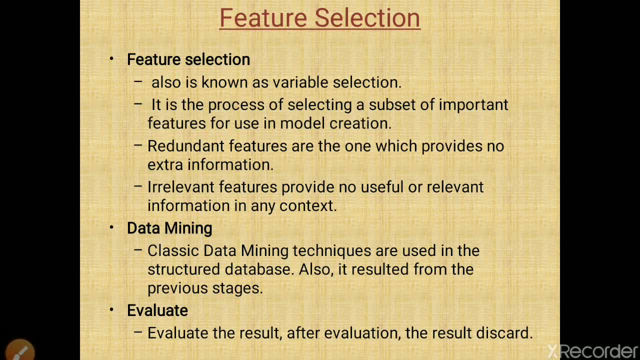 the result after the evaluation. after the evaluation, that result is stored. What is our purpose? We are doing the text mining, So we have to find a some interesting pattern after mining that. So that will be evaluated. So these are the main process. So last step in the 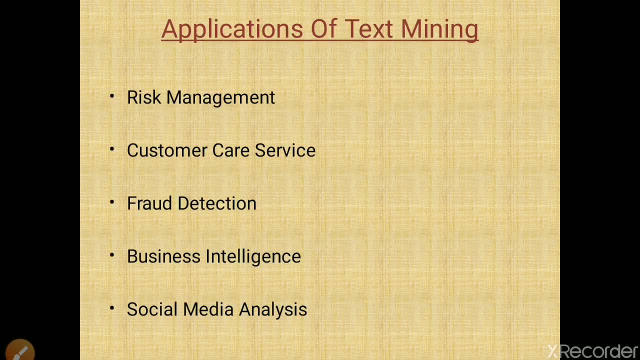 process is application. So this text mining is used in many, many areas, and some areas like risk management, customer care services, fraud detection, business intelligence and social media analysis and all Risk management in the case, if you are given with a text related with 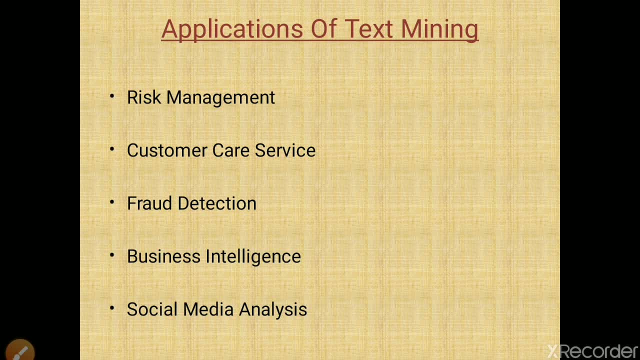 the market trend and all we have. we can analyze the text and we can find the market trend to find the risk management. Then in customer care service and all customer call transcripts are using the text mining process. So in customer care service also we are using 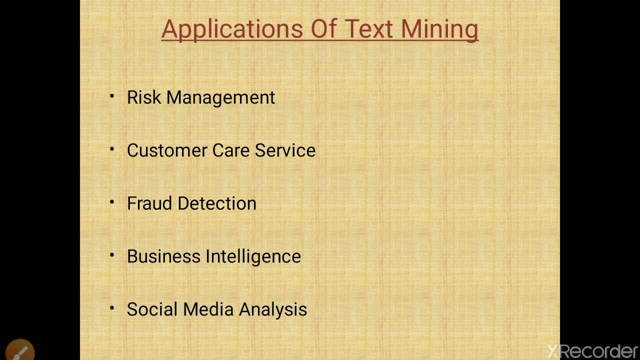 Next is fraud detection: For fraud detection and all we can use, then business intelligence. This business intelligence is like using the hidden pattern from a particular text or from a particular document. We can, you, we can use the business intelligence. And next is social media analysis: For 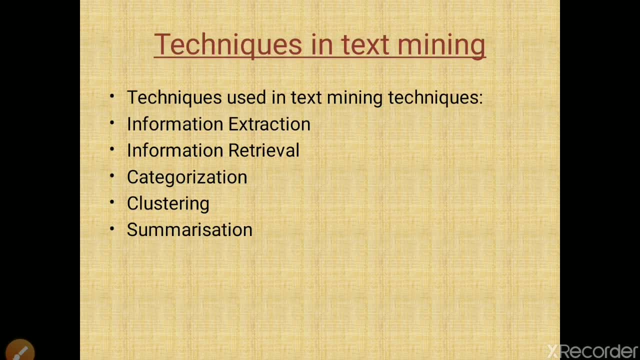 that purpose also, we are using the text mining process. Next is techniques in text mining are like. the different techniques are used for text mining process. They are information extraction, information retrieval, categorization, clustering and summarization. So these are the main techniques that we are used.